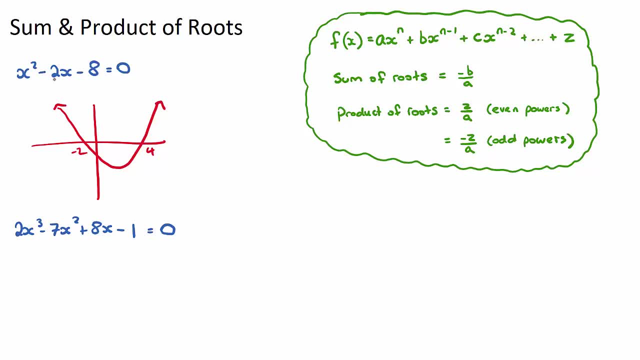 factorized it and did the null factor law, or if we graphed it on our calculator. But the sum of the roots is just summing up the two values of our roots of this equation. So that's what the sum of roots means and the product. 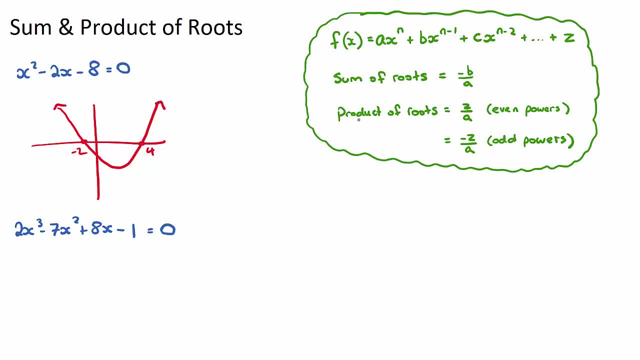 is just the multiplication of these two roots. So this is a very important topic when we look at some homework And when you're taking in yourself and the methods that we're going to go forward and do some of this. we should be looking at some. 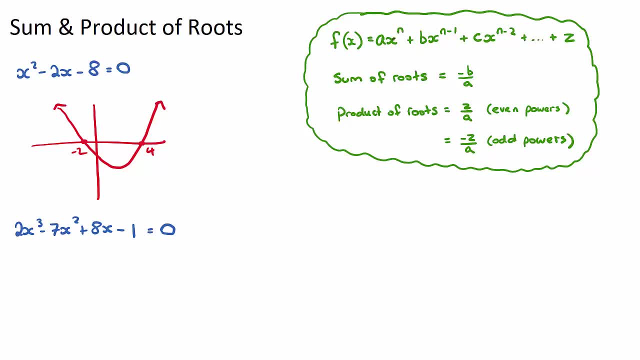 rather 잘못iveamis that we think could be able to show these three things together, All kinds of things that you did know today till the end. Okay, so we have. what are some of the solutions for this here? Well, I think. 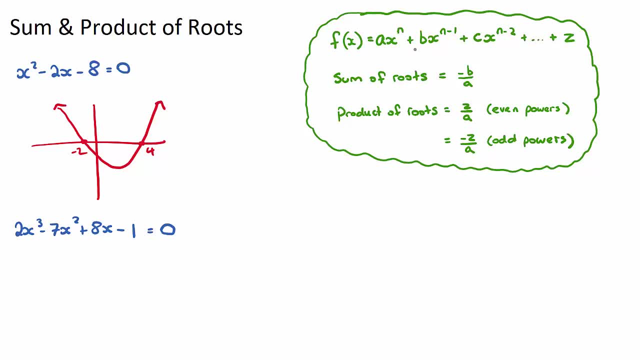 it makes sense that so perfectly well executed. you could use a website and get a lot of examples for these. 6, it's the 1, 1 below it. Now, if there's no coefficient to x, to the power of 6, if there's 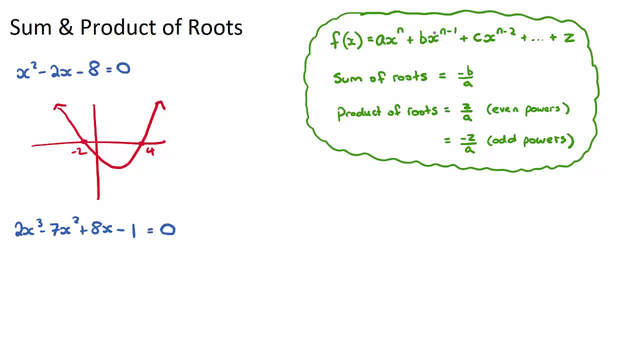 no term. the coefficient is actually 0. So we will look into that. Okay, so with our quadratic here, if we apply the sum of roots- sum of roots- the equation says it'll be negative b, so it'll be negative, negative 2 over 1, which will just be. 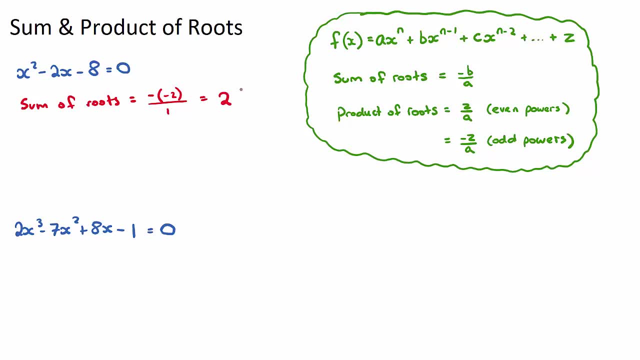 2, which is accurate to our drawing before, because our two roots were negative- 2 and 4, and if we were to sum these we would get positive 2.. Now, the product of our roots, product of roots, the product of roots formula. the answer is z on a, so it's the constant term over the coefficient. 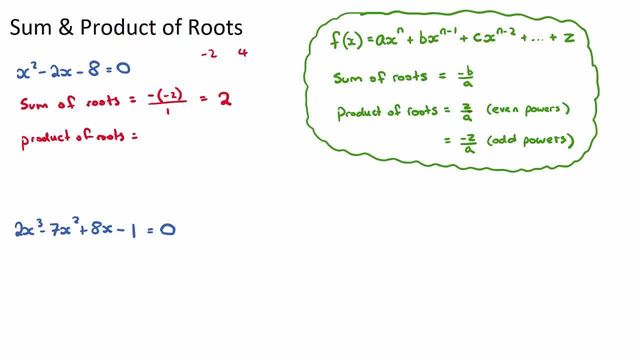 of our largest term and it's positive z on a if our polynomial has an even power, so a quadratic 0.. x to the power of 2,, x to the power of 4,, x to the power of 6, if our largest power is even. 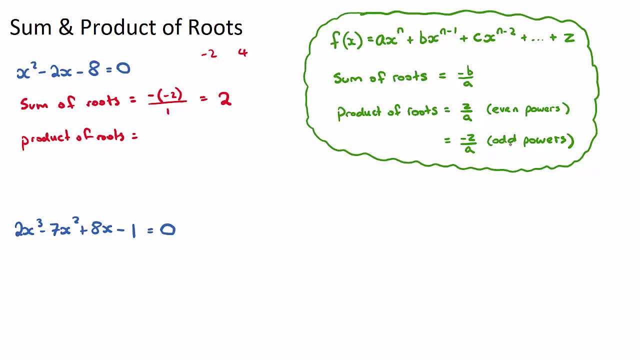 it's just z on a, and if it's an odd, for example a cubic function, it's negative z on a. So for ours it'll be positive, negative 8 on 1, so therefore negative 8, and we knew that would.